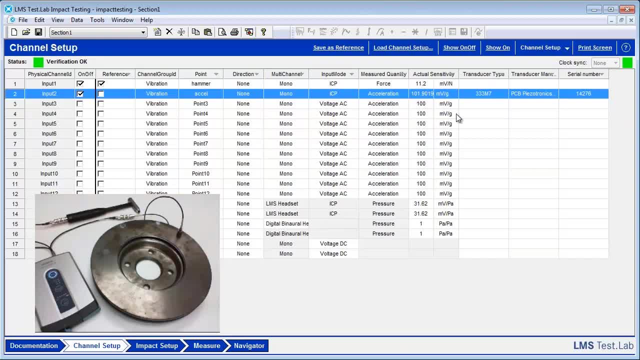 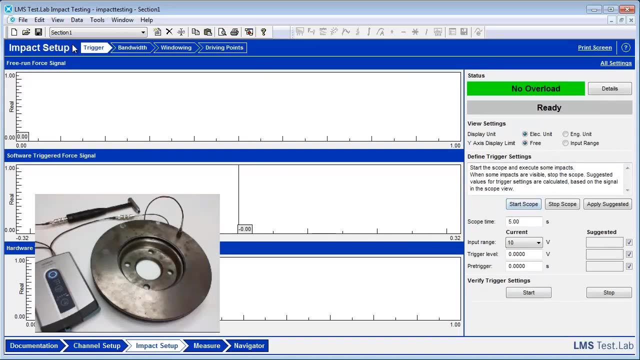 And, as you can see, Test Lab adds in the actual sensitivity for the accelerometer, tells us the transducer type and even gives us the serial number. Once that is done, we can go ahead and go to Impact Setup. In Impact Setup you can see that there are a few different worksheets here at the top. 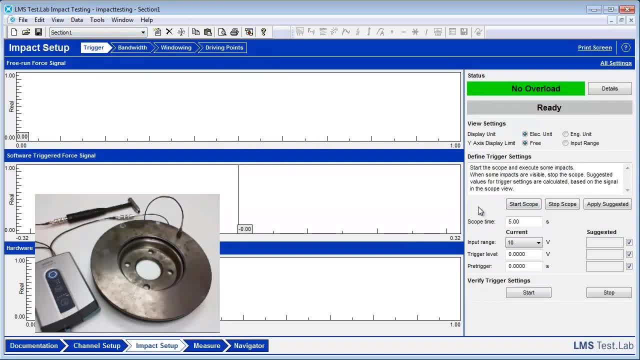 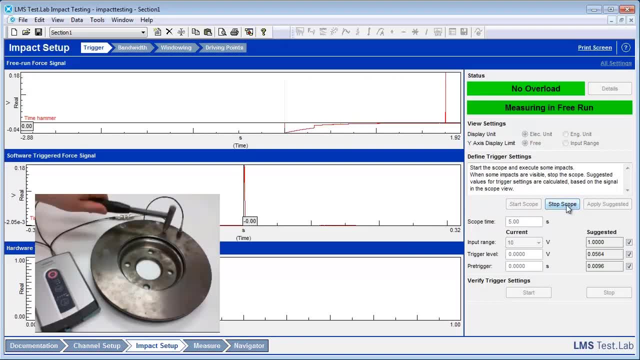 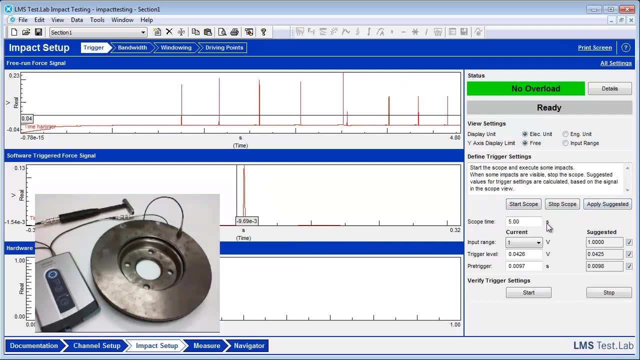 First one is going to be Trigger. This is where Test Lab is going to try to figure out a good trigger level for our measurement. We can do this by Start Scope, Hitting the object multiple times, Pressing Stop Scope And doing Apply- Suggested. 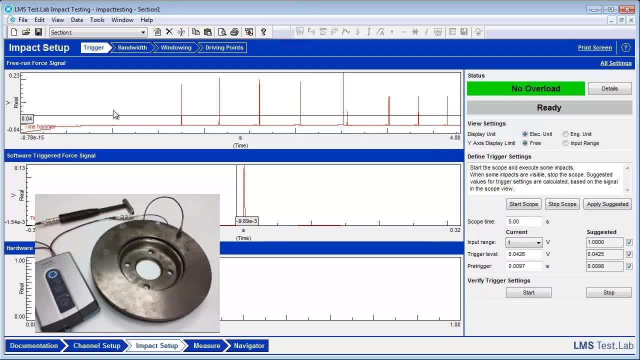 As we can see, Test Lab adds this little black line here, which is their recommended trigger level. If need be, we can come in here And manually change this. Once that is complete, we can head to the next worksheet, which is Bandwidth. 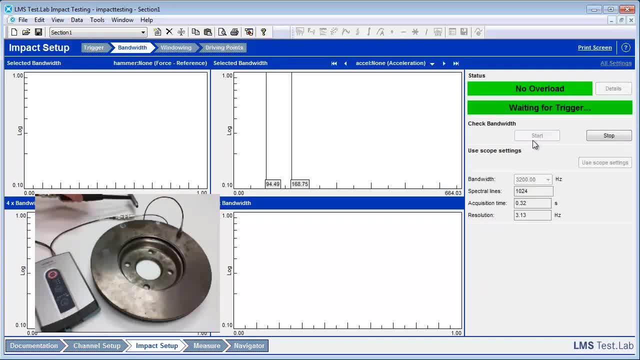 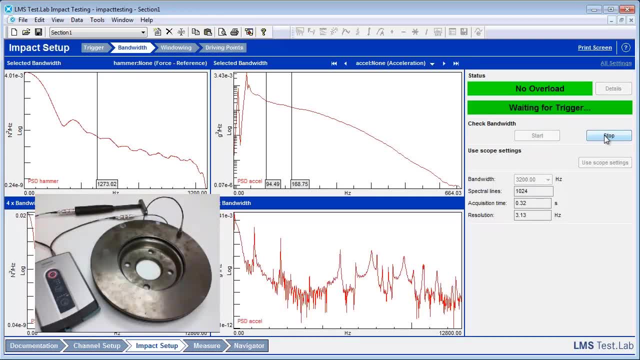 We can press the Start button And hit our object. Now, what we want to look at in the Bandwidth worksheet is this top left window. This is actually showing us the frequency spectrum for our hammer. What we want to do is switch this Y-axis to decibels. 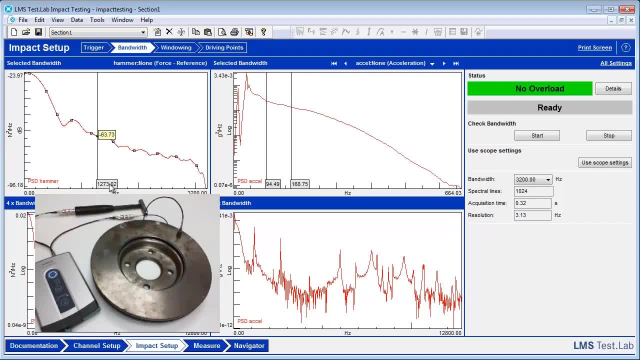 And then we want to analyze how much of a drop-off we have in this signal. Some places, some people like to follow a standard rule of thumb of no more than 10 dB drop-off. Others keep it to 3.. Regardless, this signal has much, much too great of a drop-off. 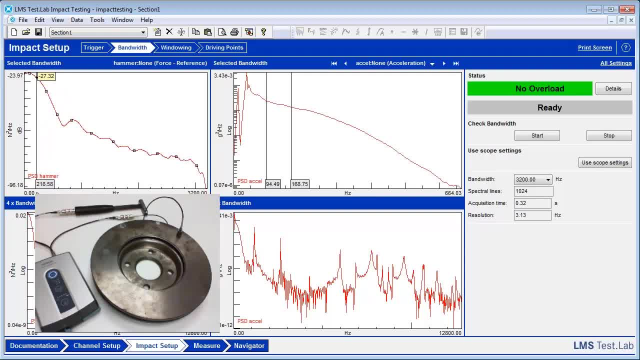 And it actually even peaks after the drop-off. What I mean by that is: you can see, this yellow tag says that this signal starts around 24.. And so then, if we took it to about here, which is our 10 dB drop-off, 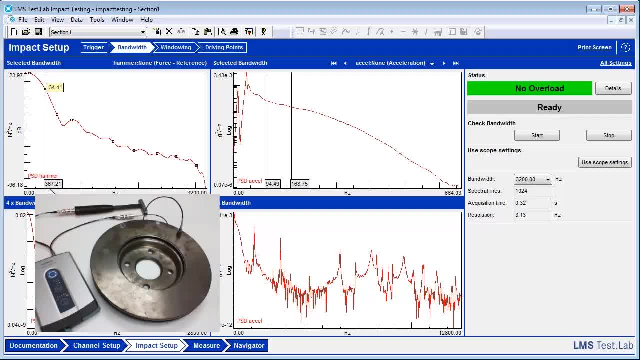 we're really only good up to a frequency of about 367 Hz, And we want to be a lot higher than that. So the first thing we can do to try to fix this is switch out our hammer tip. Right now we have a rubber tip on our hammer, which is a very soft tip. 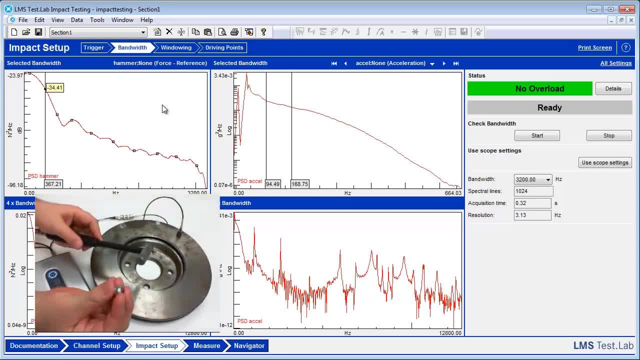 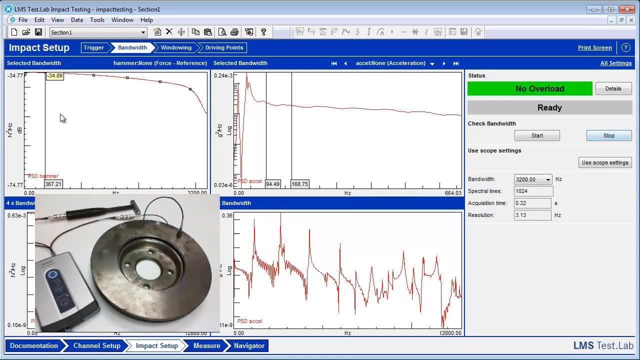 So we're going to try to switch that out for a metal tip And we're going to start our check bandwidth again And, as we can see, we get a much flatter signal across our whole frequency range of interest And we are well within a drop-off range of about 6 dB. 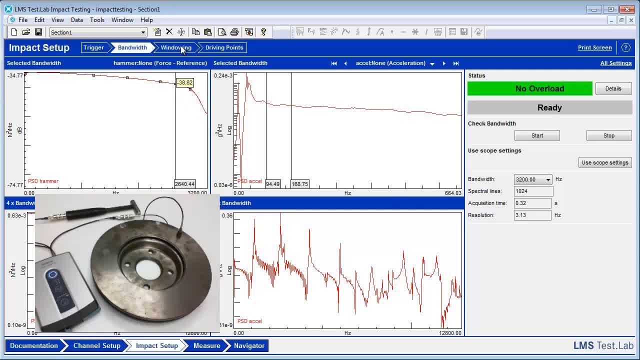 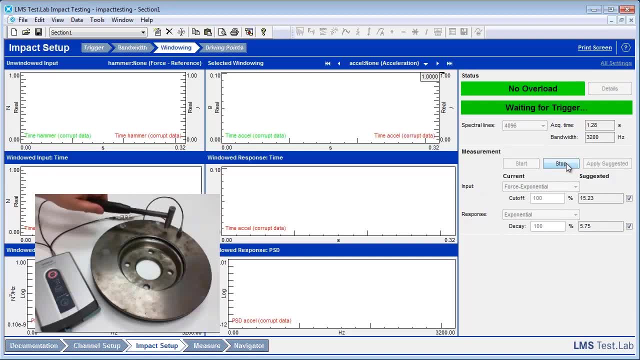 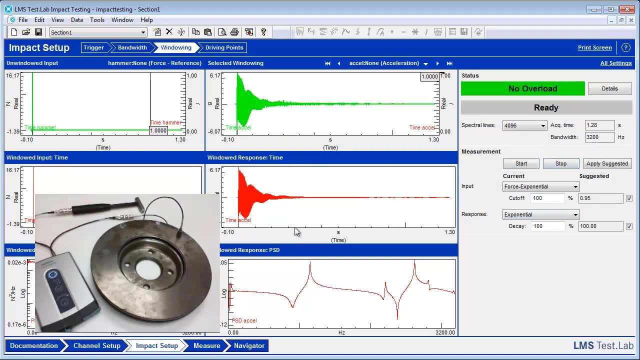 So that's good. We can go ahead and go to the windowing worksheet Here. we can go ahead and start, Impact our object And, as we can see, our signal mostly dies down within our acquisition time. So Test Lab recommended 100%, which is actually no window at all. 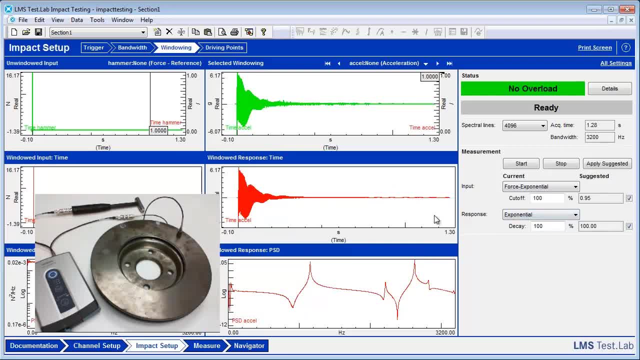 If we would like to add a window, for example, if our signal didn't die down during this acquisition time, we could come up here and drag down this line, And what this is doing is multiplying this signal here to this one, And you can see that result in this window here. 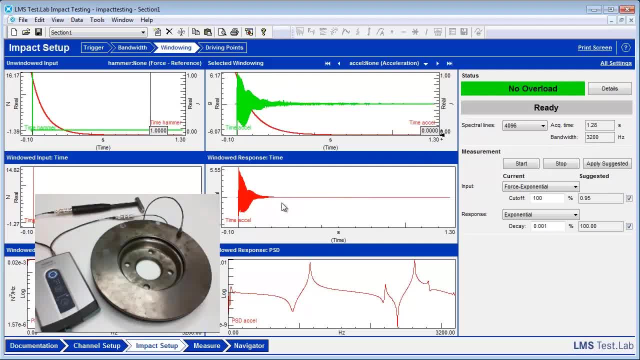 So if we were to bring this all the way down, we can see that our signal dies down much earlier in our acquisition time. So that window is adding artificial damping, which is something that we don't want. For this example, we don't need much of a window. 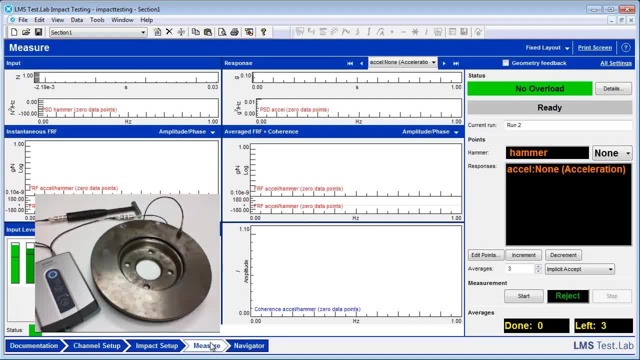 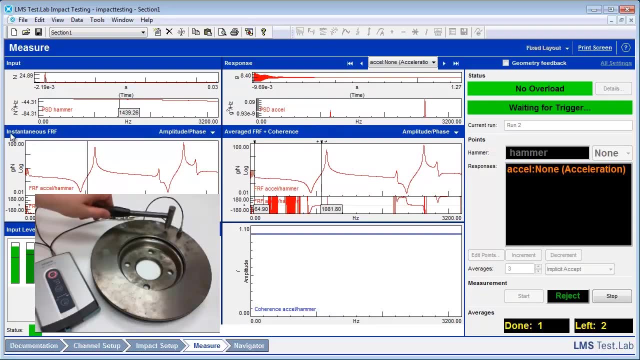 So we are ready to head over to measure. Once we're on the measurement worksheet, we can go ahead and press the Start button. During the measurement we get some displays that show up after each impact. The instantaneous FRF is going to give us a newly calculated FRF for each individual impact. 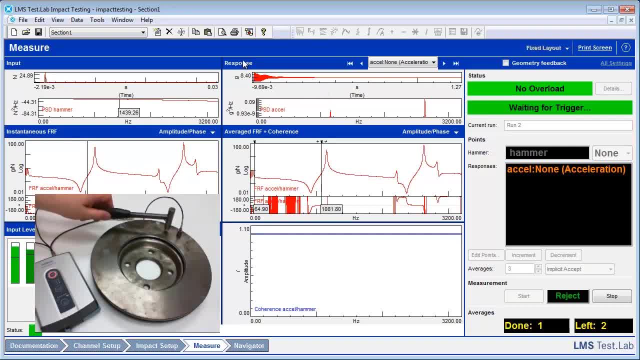 And then we can go ahead and start measuring. We also get displays that show us the response and the input in both the time domain and the frequency domain. Once we've completed three hits, as our averages are set to three, we've completed one full measurement. 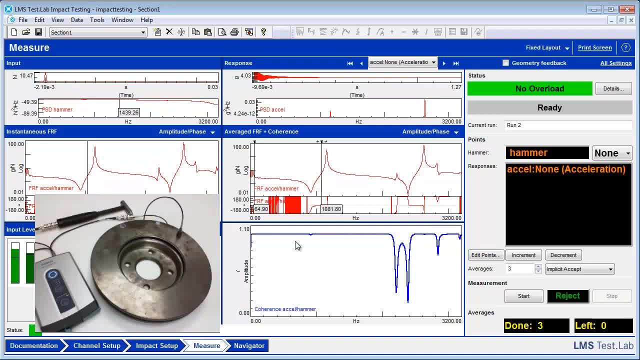 One thing we want to check is our coherence, which we see in this bottom right window here. Coherence tells us how repeatable our measurement is from hit to hit. When the coherence is equal to one, that means it's repeatable. We have a couple dips here in our coherence, but these do line up with dips in the FRF also.